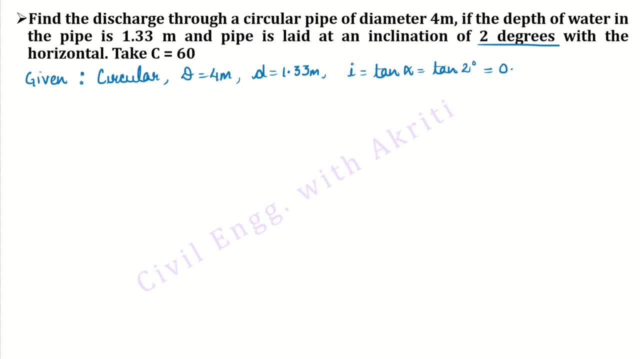 is given indirectly, which is equal to tan of 2 degrees. So i's value is given indirectly, which is 0.0349, and c has been told to us that it can be taken equal to 60. So if we make a cross section of 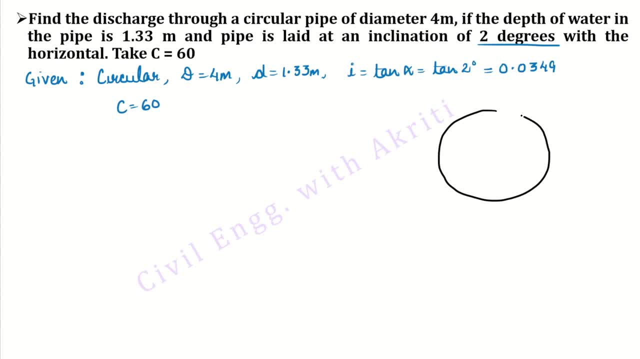 the pipe, then the pipe is circular and it is told that if it is in the center then the radius will be equal to d by 2.. So d by 2 means 4 by 2 meters, that is equal to 2 meters. So if i draw the radius, 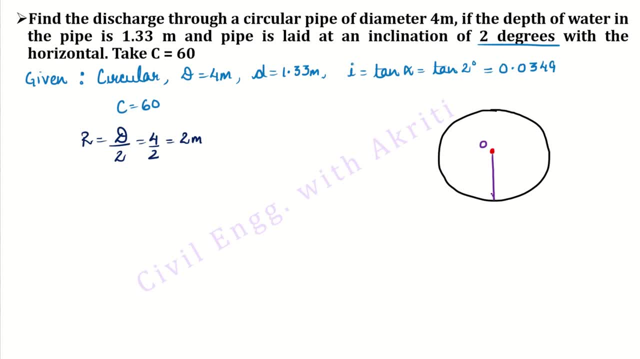 So from this point O to here, I have distance 2 meters. Now I have the depth of water given. The depth of water is equal to 1.33 meters. So I am getting to know that the depth of water is less than the radius. 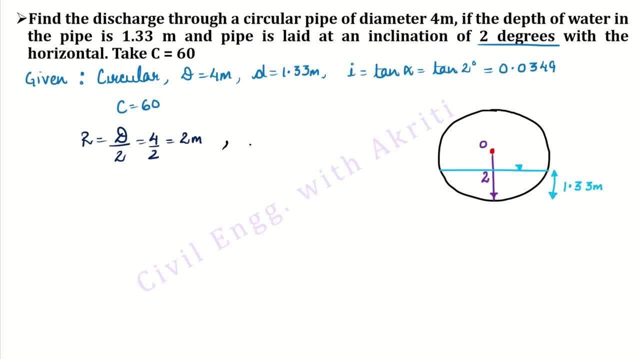 I can say that the depth of water is equal to 1.33 meters. So this is the case where radius is greater than depth of water. This is important. We will see why in the future. So we know that when we did derivation for circular section. 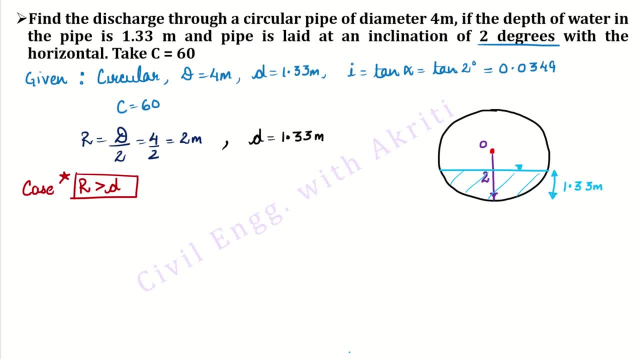 we saw that if we have to calculate the area of this shaded portion, then what we have to do is this: second, we have to calculate the area of sector ABDO. We have to calculate its area and minus the area of triangle. So area of flow is area of sector ADBO minus area of triangle AOB. 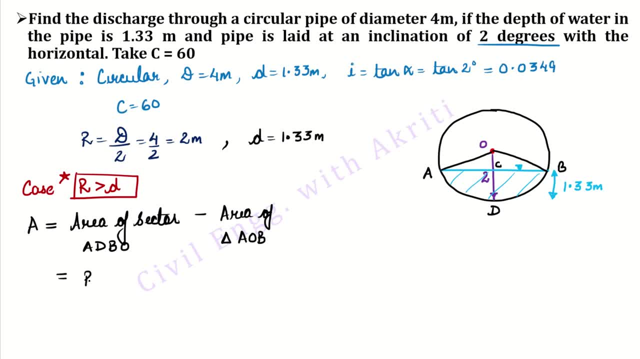 So when we did derivation for this, we got the answer. We got the answer: R square into theta minus sine 2, theta divided by 2.. This is the value of area. Now, what is it? How do we use values in this? 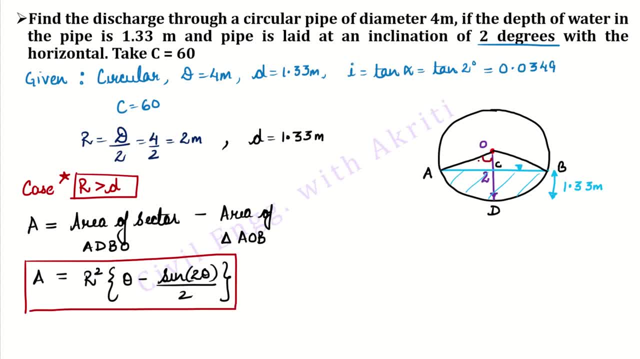 First, what is theta? Theta is this angle. What is theta angle? Angle AOC is equal to theta. Why? Because angle AOB is equal to 2 times theta. What is the angle of sector 2 theta? Now we have to see that when I will substitute values in this formula. 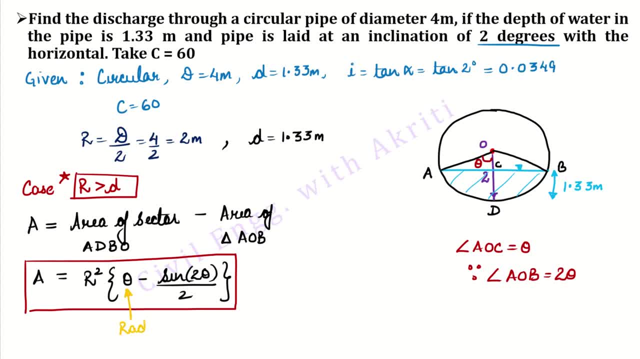 then this theta will be in radians and this theta will be in degrees. So when we calculate the value of theta, then we have to calculate in radians and degrees. Now let's talk about perimeter, The formula of perimeter. we have derived 2R theta. 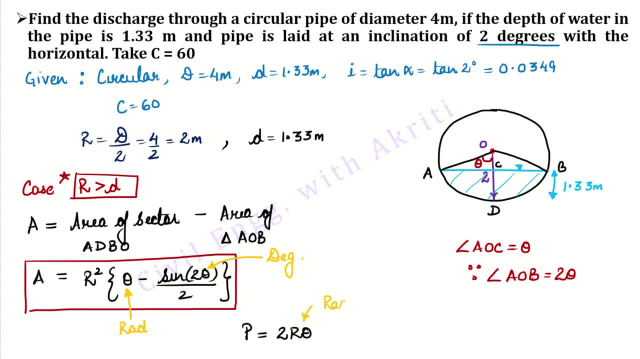 Here also, the value of theta will be in radians. So we have to keep in mind that where the value of theta will be in degrees and where the value of theta will be in radians, Where the trigonometric function is attached to theta, 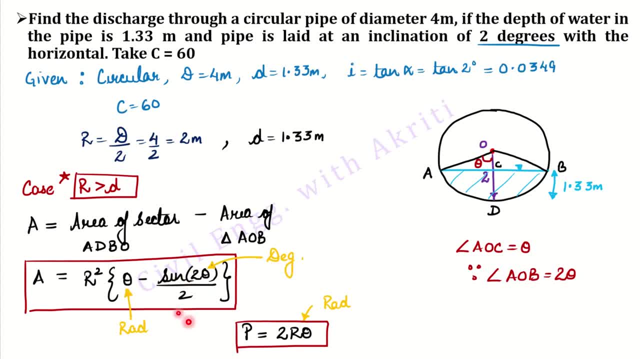 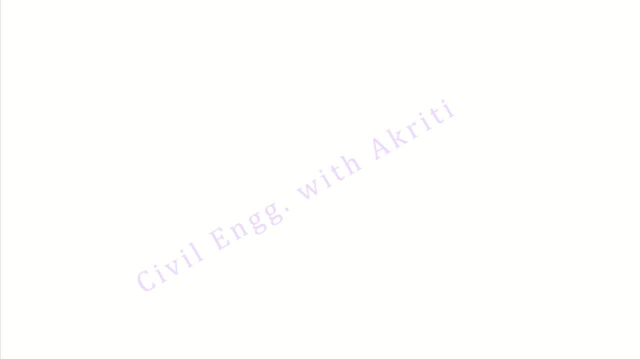 there the value will be in degrees. Where theta is alone, there the value will be in radians. So let's see how to calculate. We have a triangle, It is like this. It has O, A, B, And if we have drawn a perpendicular bisector, 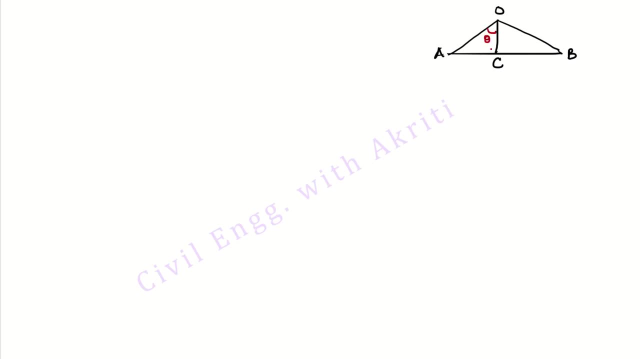 C. this angle is theta. So if I use trigonometry I can write cos. theta is equal to base upon hypotenuse. What is base? We have OC here And what is hypotenuse OA? Now we have to calculate base. 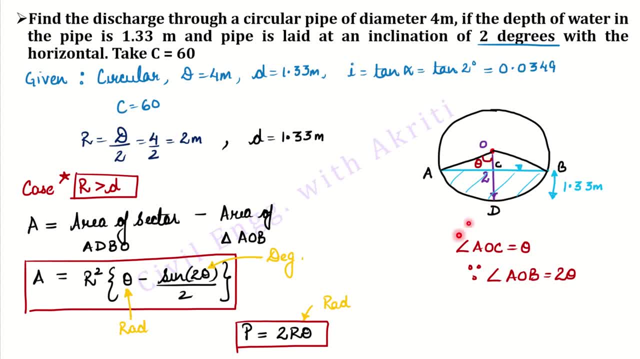 We have OC here. So how can we calculate OC? For OC? I can write: OC is equal to OD minus CD. It can be written. If we see OC, this distance is equal to OD. What is OD? It is equal to the radius. 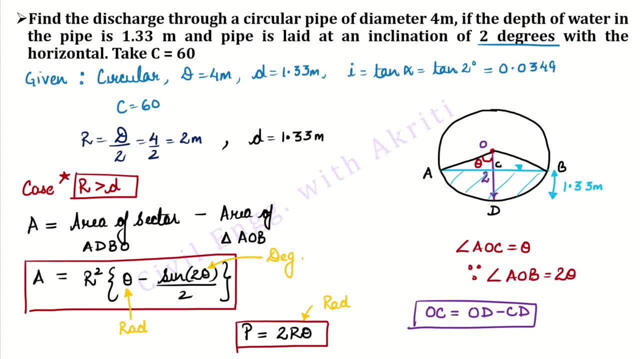 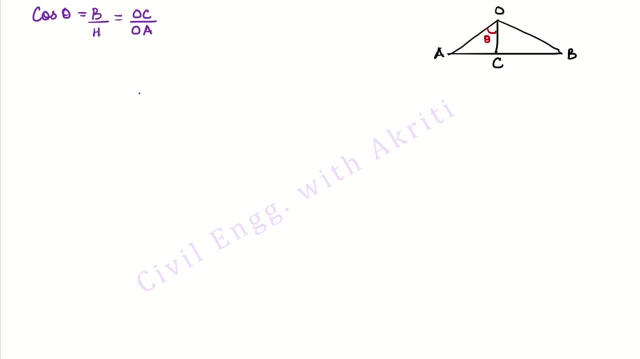 And what is CD? It is the depth of water. So I can write: OC is equal to radius minus depth of water. So OC will be equal to 2 minus 1.33 meters, which is equal to 0.67 meters. 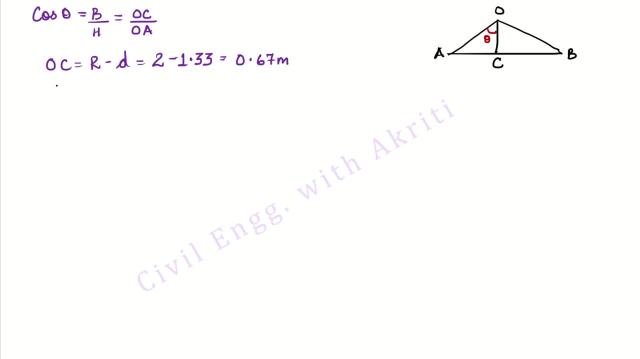 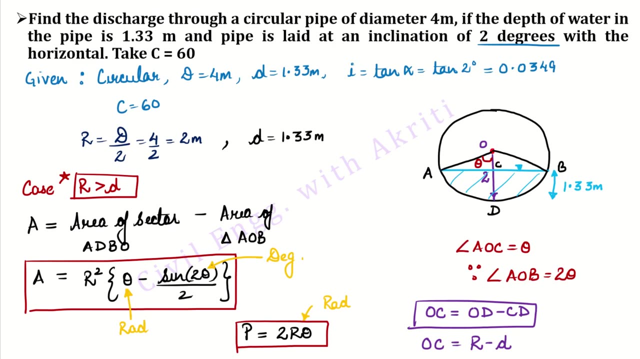 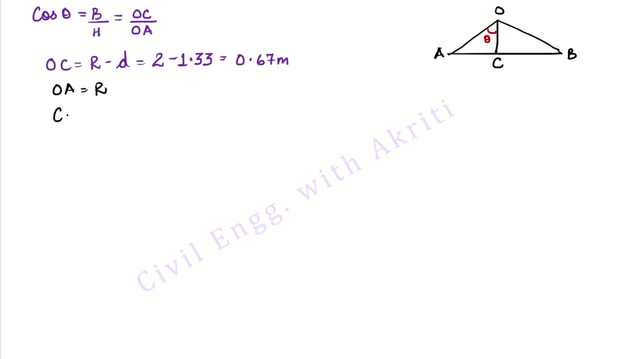 So OC's value is 0.67.. And who is equal to OA? OA is equal to the radius. If we see here, OA is equal to the radius of the circle. So I can write: COS: theta is equal to OC upon OA. 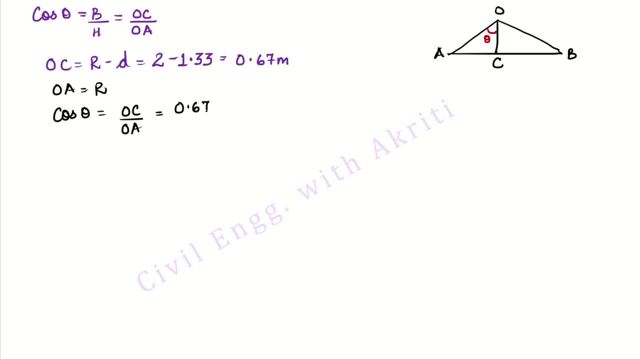 which is equal to 0.67 divided by 2. That gives me a value of 0.335.. How can we calculate theta COS inverse of 0.335.. Now, when I calculate this, I get the value of 70.43 degrees. 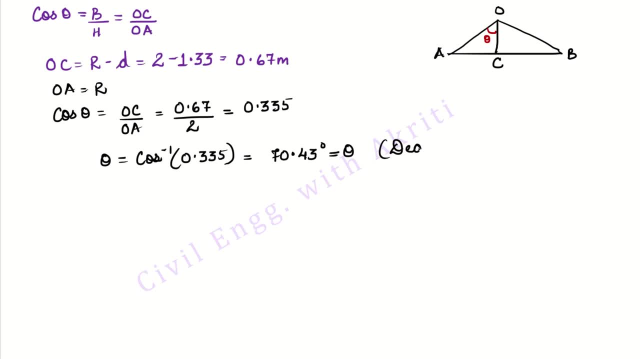 This is the value of theta in degrees. Now in which we have to calculate this, We have to calculate this in radians. So how can we calculate theta in radians? We will multiply the value of theta in degrees by pi, by 180.. 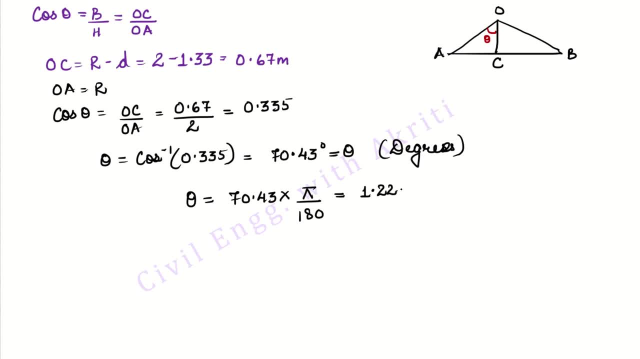 So I will get a value of 1.229 radians. So what will be the formula of area? Area will be equal to R square into theta minus sine of 2 theta divided by 2. So R square is equal to. 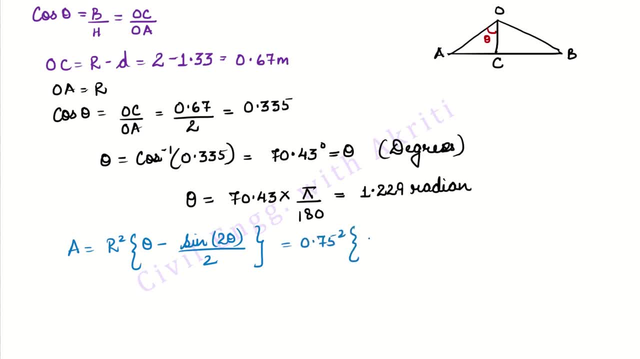 0.75 square, Theta's value in radians will be 1.229, minus sine of twice of 70.3 degrees. So we will get a value of 0.43 divided by 2.. So when we simplify this, 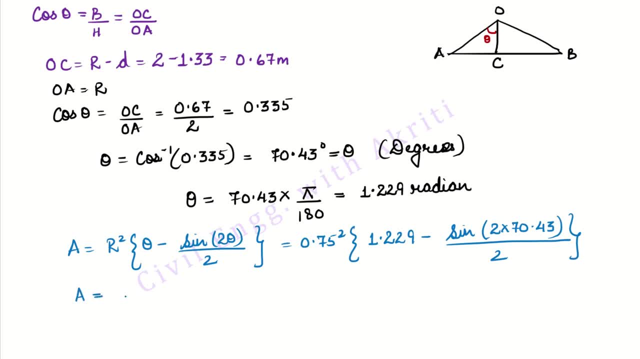 you will get the value of area equal to 3.653 meter square. This is the value of area. Now we can calculate the value of perimeter. Perimeter was equal to 2R theta. Here theta will be in radians. 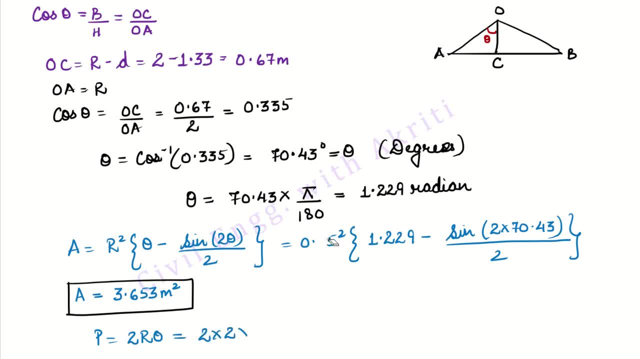 What is the value of R? What is the value of R? I am sorry, The value of R is here Equal to 2.. So into 1.229.. So that gives me a value of 4.916 meters. 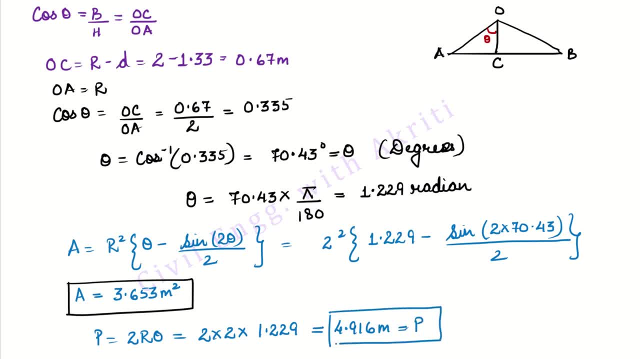 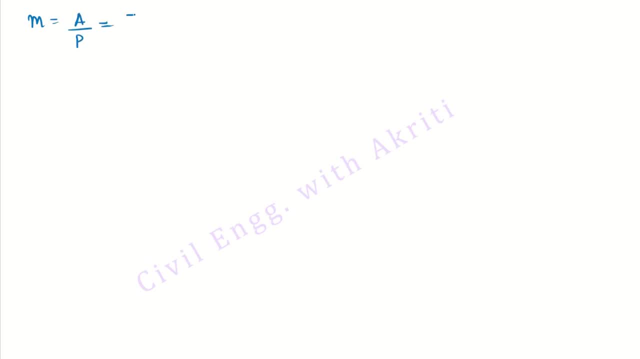 So that is the value of P. Now how can we get M? How can we get M? M is equal to area of upon wetted perimeter. Area was equal to 3.653 and perimeter was equal to 4.916. 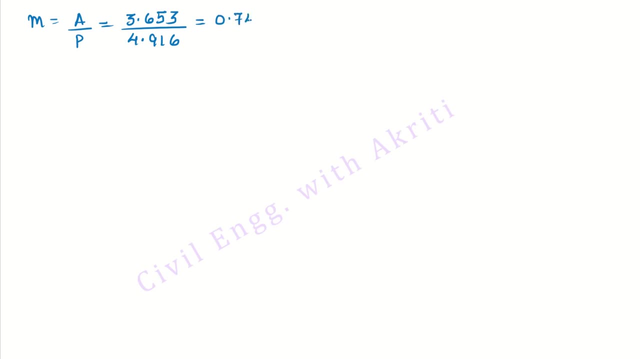 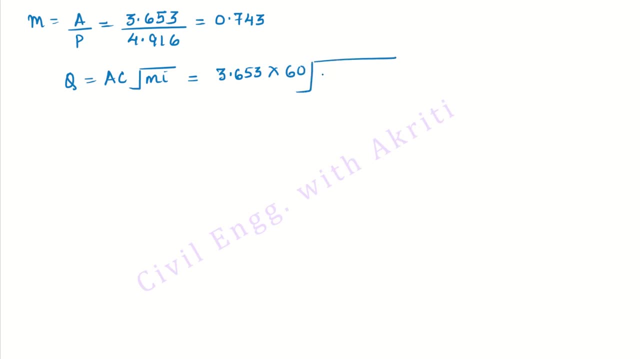 So that is the value of M Under the root of M. M is equal to: M is equal to 0.743.. I is equal to tan of 2 degrees, which is 0.0349.. So this is calculated as. 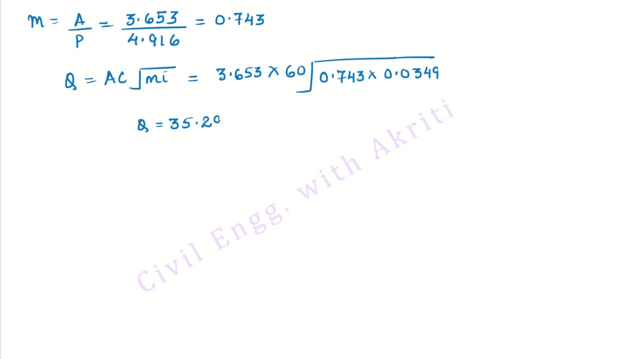 equal to 35.29 meter cube per second. This is the required answer Now. next is Next question. a culvert with a circular cross section of diameter 1.5 meters has a bed of 6 meters in 4 kilometers. 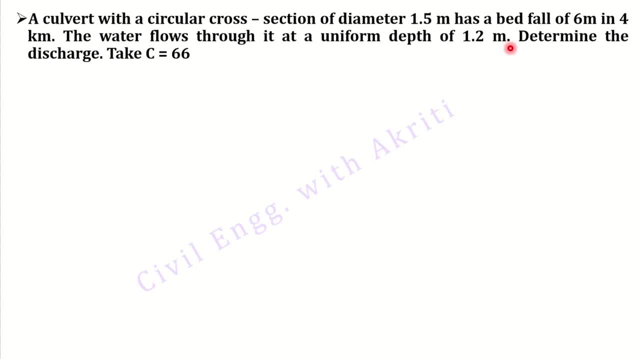 The water flows through it at a uniform depth of 1.2 meters Determine the discharge. take C is equal to 66.. So this question is very important. We are going to understand a concept in this. that's why it is important. 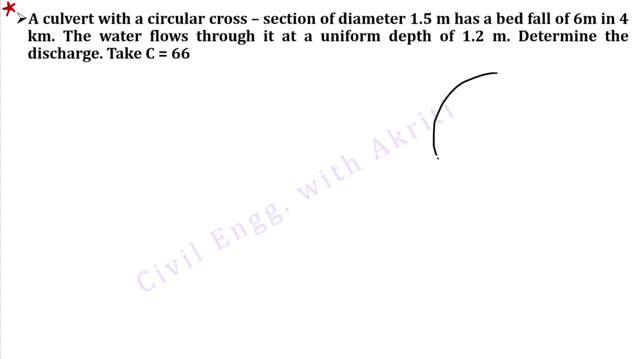 Otherwise calculations are simple. So when we are drawing a circular section, first we are given that: how is the section? it is circular. So section is circular, its diameter is 1.5 meters. Then we are told that bed fall. bed fall means slope. i is 6 meters upon 4 kilometers. 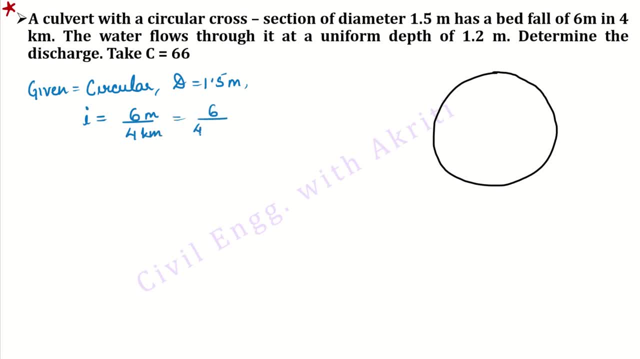 6 meters in 4 kilometers, which is equal to 6 meters. 6 meters in 4 kilometers, which is equal to 6 meters upon 4000 meters. So this is the value of. i Depth of flow is equal to 1.2 meters and Chezy's constant's value is given 66.. 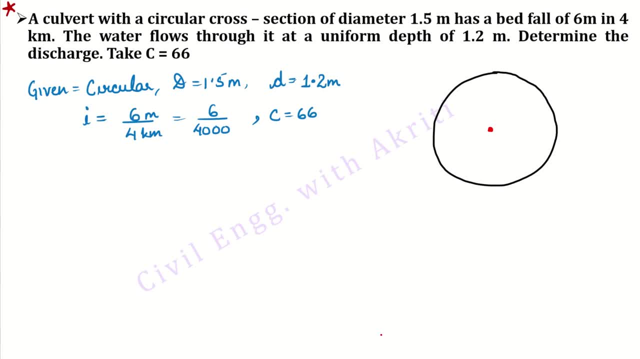 So if I assume the center of this pipe here, then I can see that its total depth is 1.5 meters. And what will be the radius? Radius will be equal to 1.5.. Radius will be equal to 1.5 meters divided by 2, which is equal to 0.75 meters. 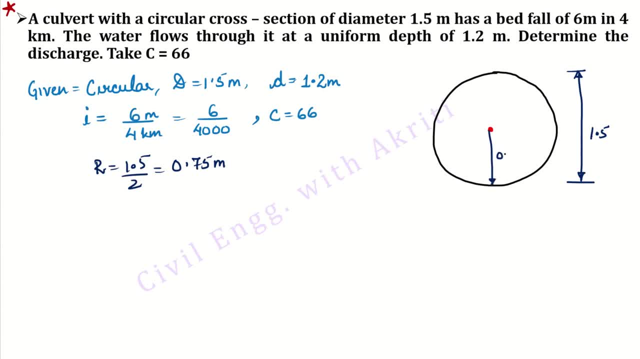 So this value is equal to 0.75 meters. So we can see that here case 2 is coming. Why is case 2 coming? Because the radius is smaller than the depth of flow. Radius is 0.75 and depth of flow is 1.2 meters. 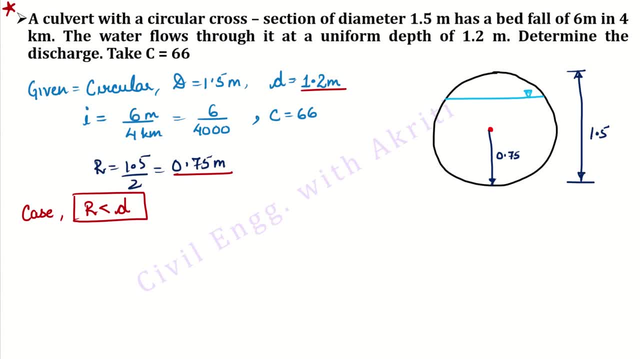 So where will my depth of flow come At this point? And this depth of flow is equal to 1.2 meters. So which area do I have to calculate? I have to calculate this entire area, So this is important. 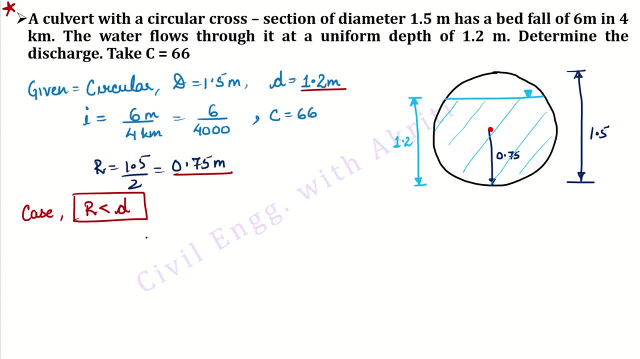 Now we know that if we have to calculate all this and use Chezy's formula, then Chezy's formula is equal to Q. If I modify it for discharge, Q is equal to A, So A is equal to V, So A is equal to C under the root of M into I. 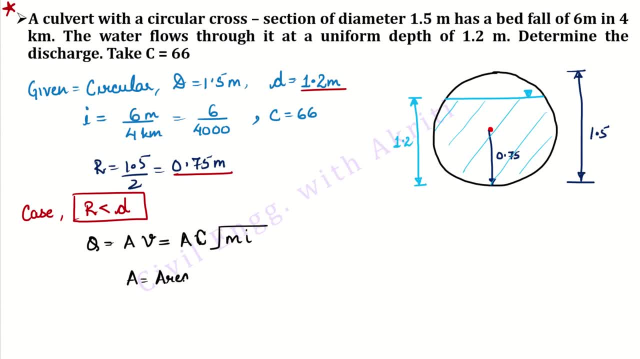 What is A Area of flow? What is the area of flow? This is the entire area that we have hatched. And what is the perimeter? What is P A by P? So P is equal to perimeter, which is the wetted perimeter. 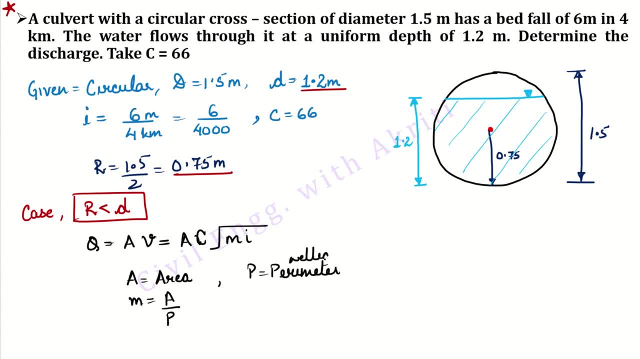 Okay, So we have to calculate this wetted perimeter. Now, what is here? When we derived the equation, so while deriving the equation, we assumed that the water level was below the center of the pipe. Now the water level we have is above the center of the pipe. 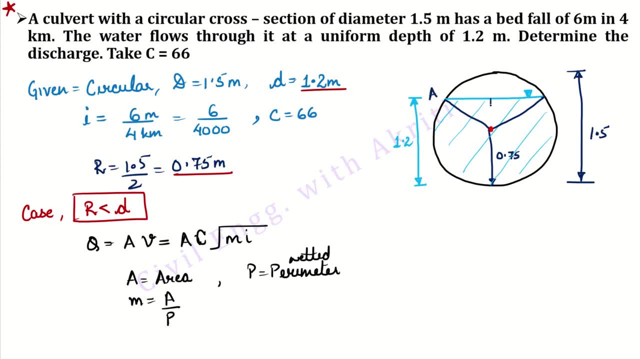 So I can give it a name: A, This is C, This is B And this point is point D. So what do we have? We have the area to be calculated. that area is equal to area of, if I give this point a name, E. 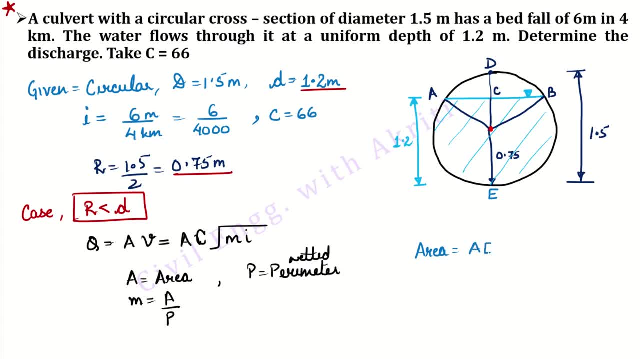 then I have to calculate the area A, E, B, C, A. Which area do I have to calculate? A, E, B, C, A? So let's see why this case is different and how we can utilize this. 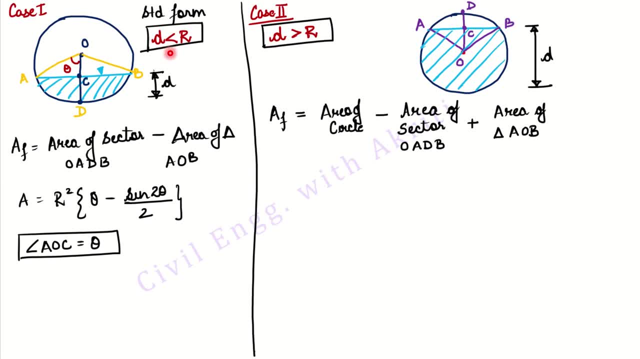 So, brief recap. We have discussed case 1, when we have derived the formula for area, What was there in that? The center of the pipe? we used to take the water level below that. So what did we do? We calculated area of sector O, A, D, B. 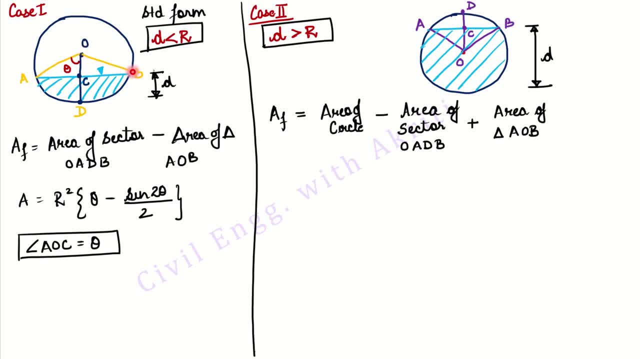 And what did we minus from that AOB Triangle area, AOB we minused Ultimately. I used to have this hatched area. We calculated its formula: R square theta minus sin 2, theta by 2.. And what was the value of theta in this case? 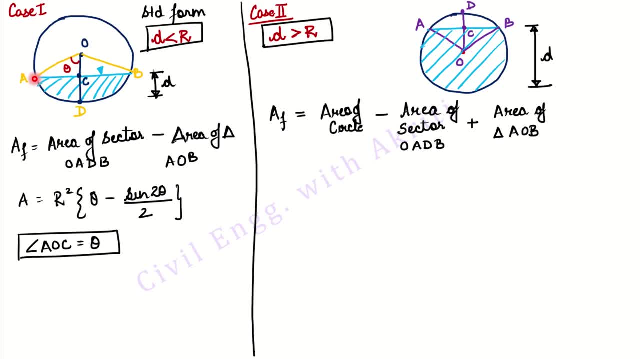 Theta was equal to this value. angle AOC, Or I can say angle BOC, This was also equal to theta. Now, what is this case? When was this case? When D depth of flow is less than the radius of the cross section? 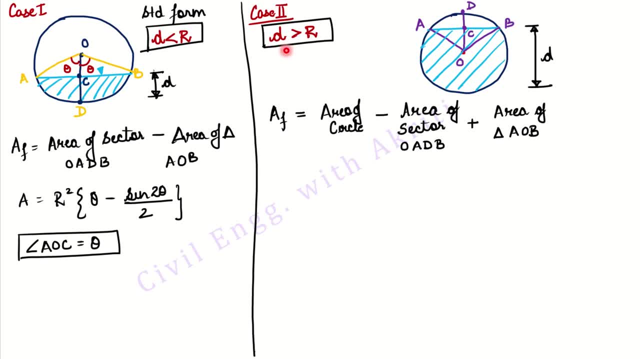 or radius of the circular pipe. In this case, what is given to us? The depth of flow D is greater than the radius of the pipe. So what do we have? How can we calculate this If we see, what can I minus from this whole area? 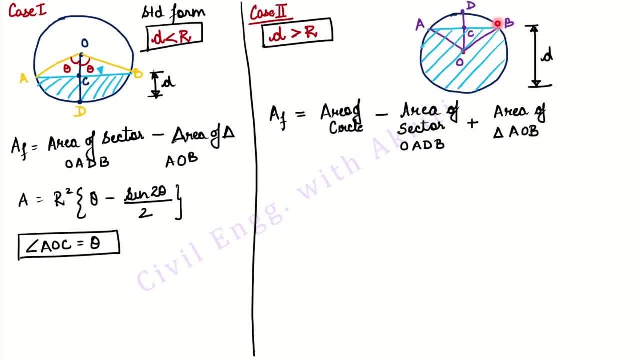 the circle area, I can minus the area of this sector AOBD. When I minus the area of this sector, I also minus the triangle of water. So what will I do? I will add it, So adding area of triangle AOB. 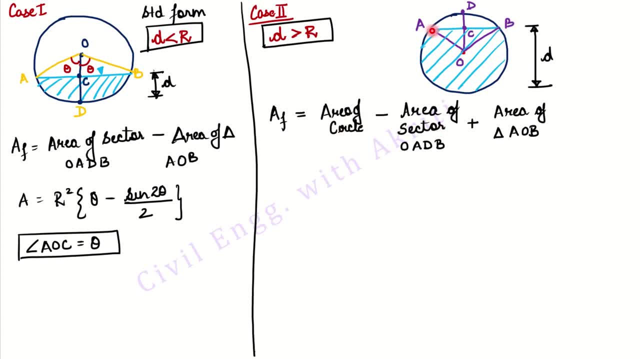 So I have to write the equation: area of circle minus area of sector OADP, plus area of triangle, AOB. So let's write the formulae For each of these terms. what will be the area of the whole circle? 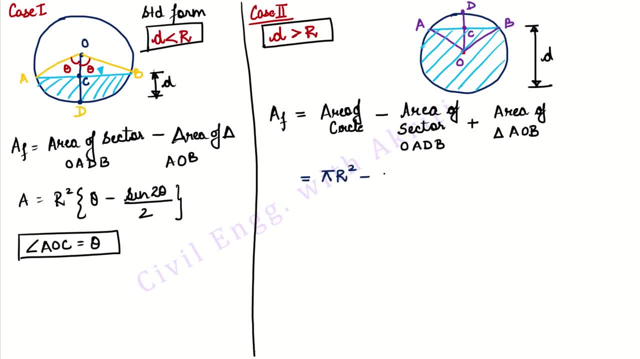 Pi R square. What is the area of sector? Pi R square into 2 alpha upon 2 pi, Okay, Plus. what will be the area of triangle In this case? what is the term alpha? Alpha is this angle. This angle is known as alpha. 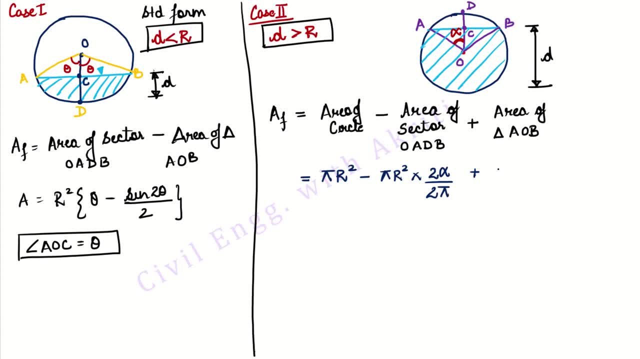 So what will be the area of triangle? Area of triangle will be equal to R square sine of 2 alpha divided by 2.. When we were doing the derivation in hydraulic mean depth, we have calculated this. So here it is very important that 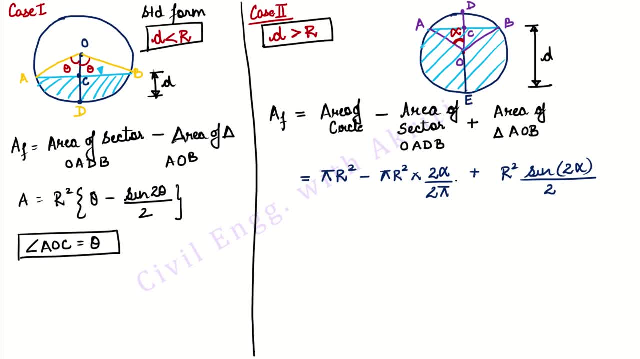 if I call this value as E, then why have we used alpha? We have used alpha because what is the sector? We have sector AOBD. What is its angle, Alpha, And which is theta angle, This remaining angle, what will we call it? 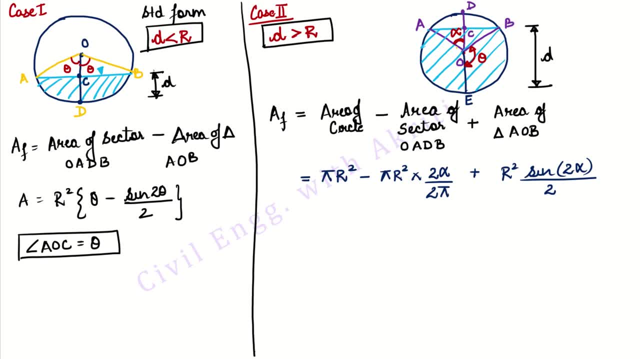 This angle will be equal to theta, So this angle is also theta, This angle we have, we are calling it theta. And this angle, DOC will also be equal to alpha, So I can write angle AOC. This is point C. 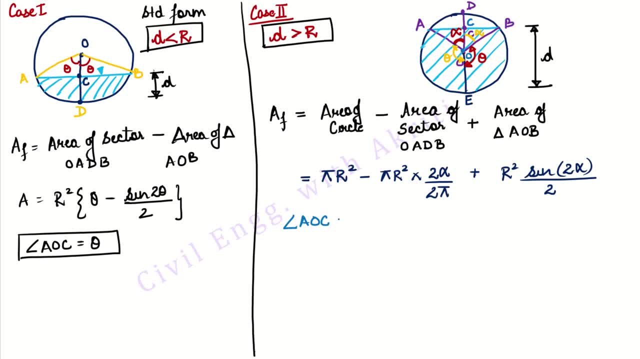 This is point O. Angle AOC is equal to angle, BOC is equal to alpha. That is why: what term have we used here? We have used alpha. And what can we say? Angle AOE is equal to angle BOE, which is equal to theta. 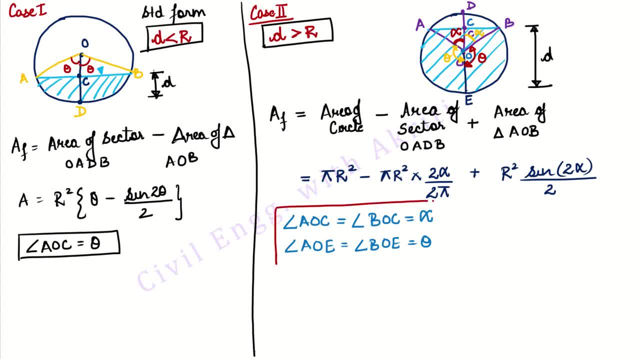 It can be said So, to memorize these angles, to understand these angles, it is very important that how we have taken angle alpha and angle theta. Now, what can we see? We can see that what is DCOE? It is a straight line. 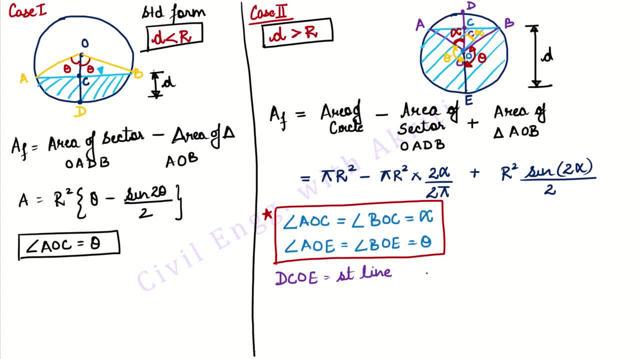 If DCOE is a straight line, then what can we say? Alpha plus theta is equal to pi. Pi means equal to 180 degrees. What can we say? This angle plus this angle's sum will be equal to 180.. So we have one more equation. 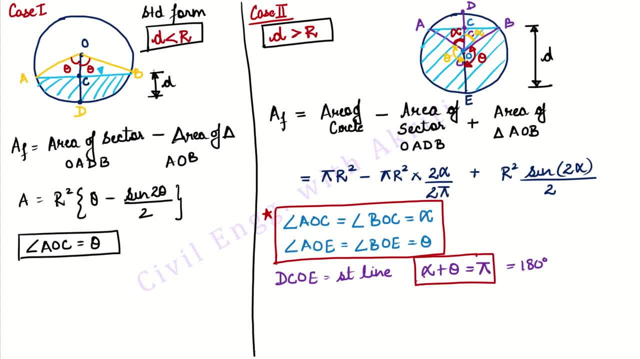 Alpha plus theta is equal to pi Clear. Now, if I see here, I can cancel 2 from 2.. And now we will leave pi r square as it is. Let's simplify this equation: Area of flow is equal to pi r square. 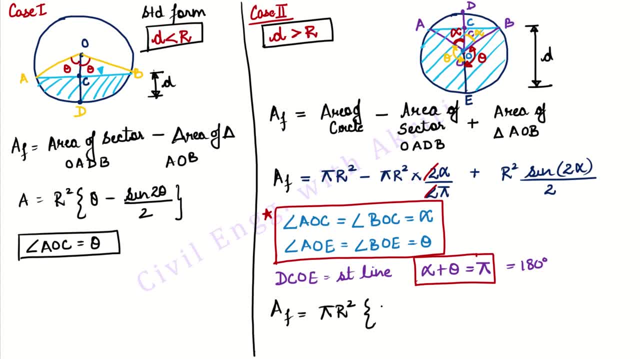 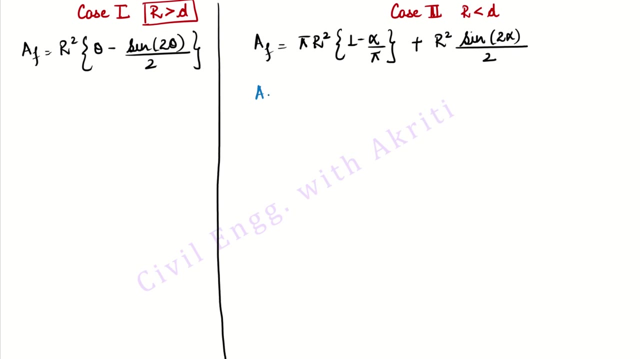 I can take pi r square as common. I have taken pi r square as common. Now I get 1 minus alpha upon pi plus r square, sin of 2, alpha whole divided by 2.. When I simplify this so I get pi r square. 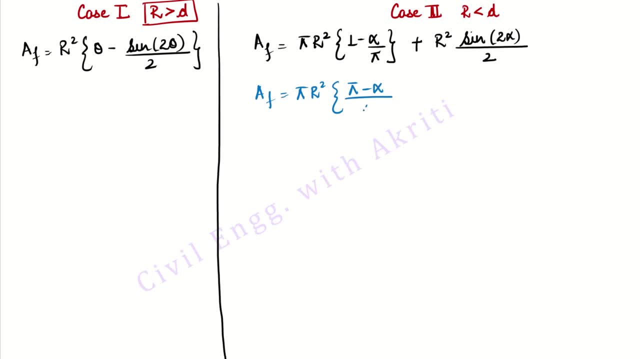 let's take LCM: Pi minus alpha, whole divided by pi plus r, square sin 2 alpha. How can we write sin 2 alpha? It can be written as 2 times of pi minus theta. We can write like this because alpha plus theta is equal to pi. 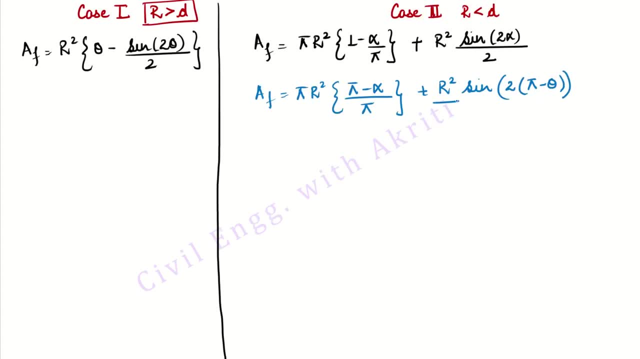 So how did we write alpha, Pi minus theta? This is divided by 2.. Now we know that because theta plus alpha is equal to pi. so we can say pi minus alpha will be equal to theta. So I can write: 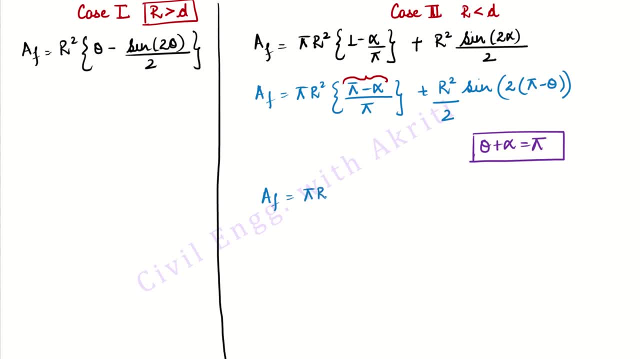 area of flow is equal to pi r square into theta by pi plus r square by 2. sin of 2 pi minus 2 theta. Can you write: I have multiplied 2 inside, So this pi gets cancelled With this pi. 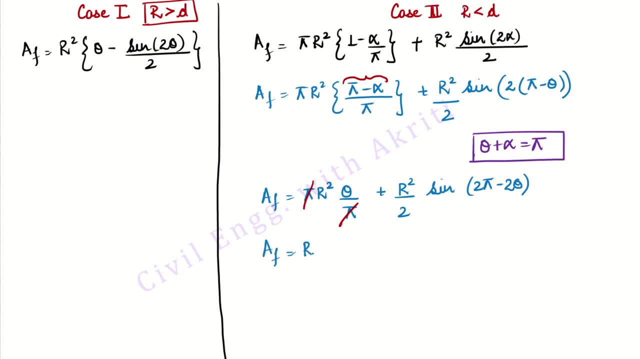 I am left with. area of flow is equal to r square theta plus r square by 2.. Now sin 2 pi minus delta is equal to minus of sin delta. Where did this come from? Because now sin has gone to which quadrant? 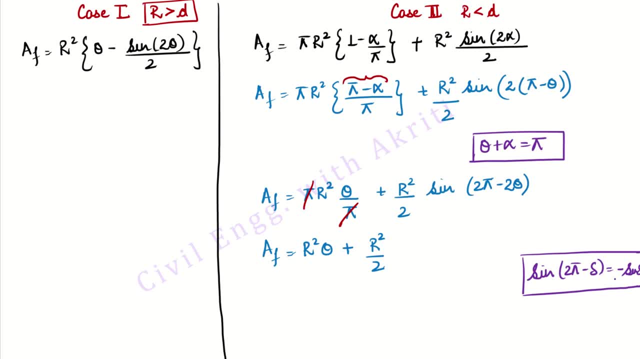 Sin has gone to fourth quadrant where sin can be written as minus sin delta. So I can write here: sin of 2 pi minus 2 theta can be written minus of sin 2 theta. Now, if we simplify this then we get: 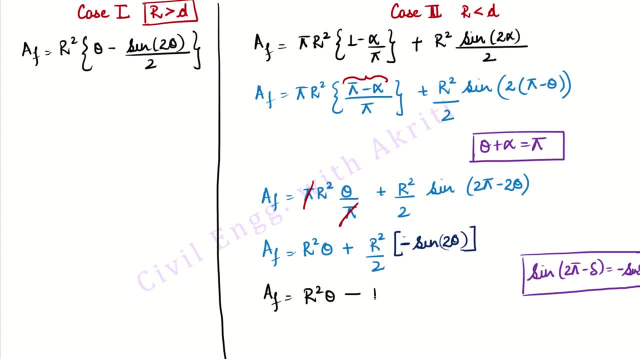 r square theta minus of r square sin 2 theta divided by 2.. If we take r square common, then I am left with theta minus sin 2 theta divided by 2.. If we see then this formula, it resembles the formula. 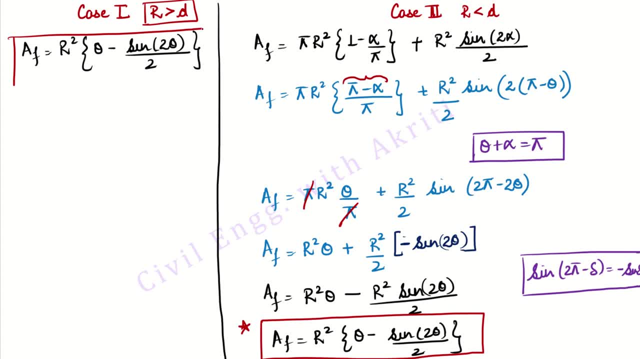 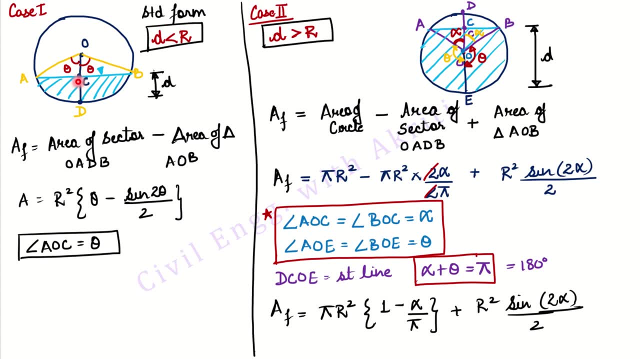 which we derived for case 1.. So with this we can understand from the whole derivation that whether your water level is below the center of the circular section or above the center of the circular section, the formula of area of flow will remain the same. 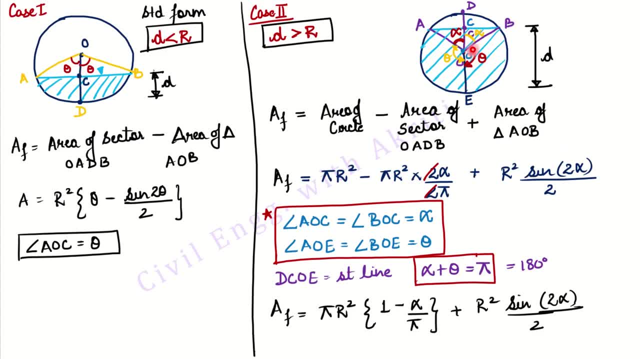 Only how to select the value of theta. that will be changed Theta here this angle is AOE or we can say BOE, And here theta is angle AOC. So it is important that how to select theta in both cases. 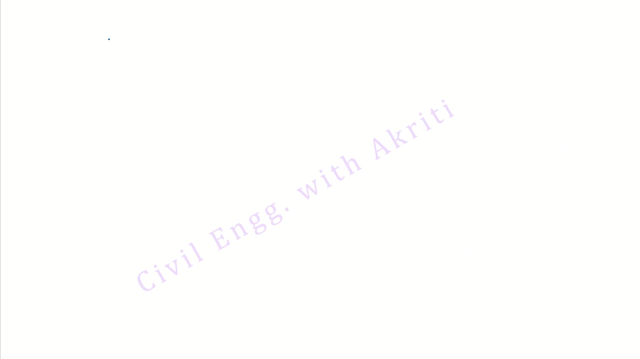 So now let's come back to our question. In the question we have given the diameter 1.5 meters. i is equal to 6 by 4000,, d is equal to 1.2 meters, So r is equal to 1.5 divided by 2,. 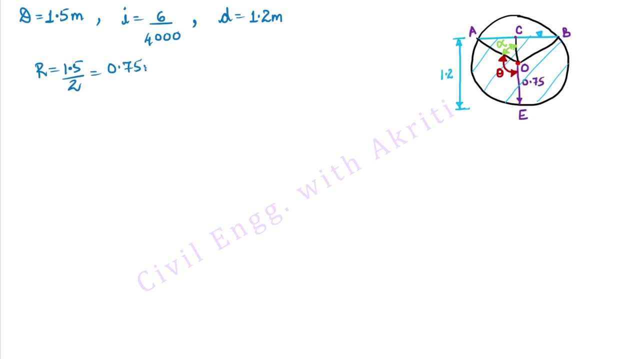 which is equal to 0.75 meters. We have the formula of area of flow r square into theta minus sin 2 theta divided by 2.. So first let's calculate theta. theta is equal to pi minus alpha. So what will I have to calculate for that? 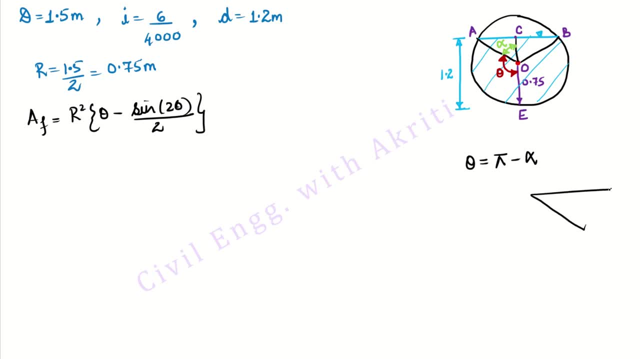 I have to calculate alpha. How will we calculate alpha? I have this triangle. This triangle is ACB and this will be O, So alpha will be equal to. if I talk about cos alpha, cos alpha will be equal to OC upon OA. 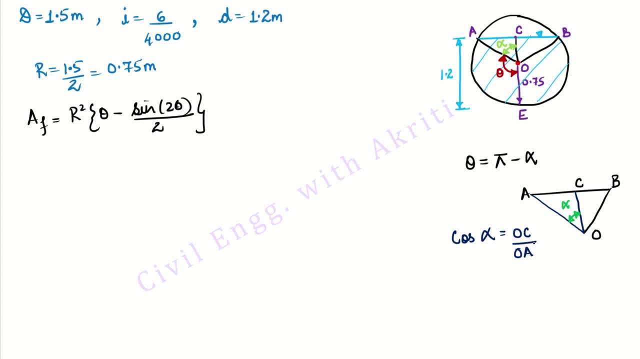 Base is OC and hypotenuse is OA. So how can OC be calculated? OC is equal to CE minus OE. What is CE? CE is the depth of water, small d, and OE is the radius of the circle, which is equal to 0.75.. 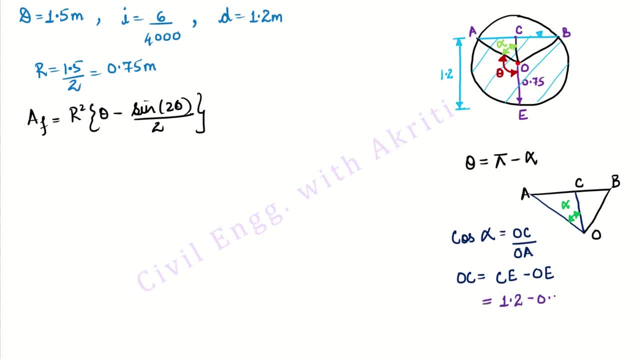 So 1.2 minus 0.75, which is equal to 0.45.. So this is 0.45 meters. So how can we write cos alpha? cos alpha will be equal to 0.45 upon 0.75,. 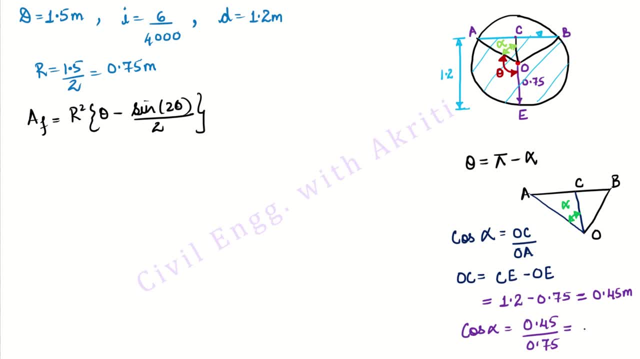 which is equal to 0.6.. So we have cos alpha. alpha will be equal to cos inverse of 0.6.. which is equal to 53.13 degrees. So what did we have to calculate? We had to calculate theta. 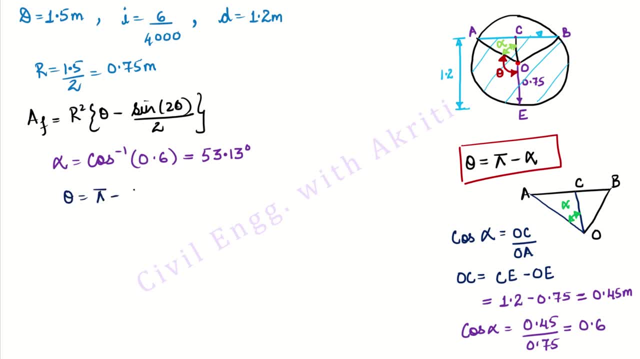 theta is equal to pi minus alpha. So what can I write pi minus alpha? pi minus alpha is 180 degrees minus 53.13 degrees, Because alpha is also in degrees. so what did I write pi in? It is written in degrees. 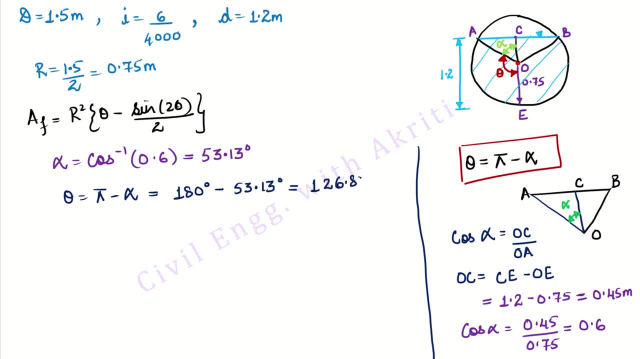 That is equal to 126.87 degrees. So theta is equal to 126.87 degrees. And how can we convert this into radians? into pi by 180, which will give me 2.214 radians. So this is the value of theta in degrees. 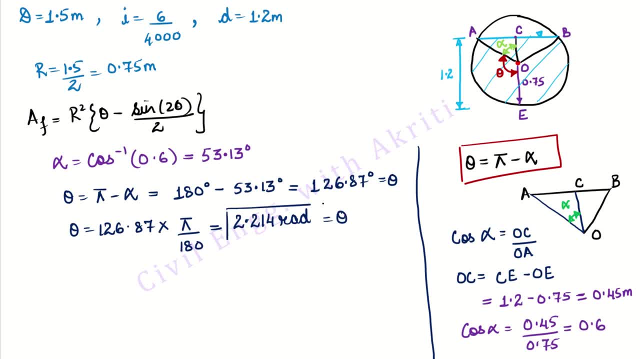 and theta in radians. Now I can substitute this in the formula of area. So let's do that. area is equal to r. square is 0.75 square. theta in radians is 2.214 minus sin of 2 pi. 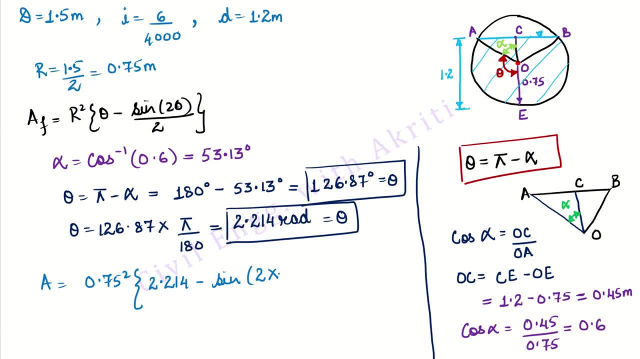 2 pi is 2 theta. theta is in degrees, here 126.87 divided by 2.. Now, if we see, then this will be calculated around 253 degrees. 253 degrees means the value of sin will be negative. 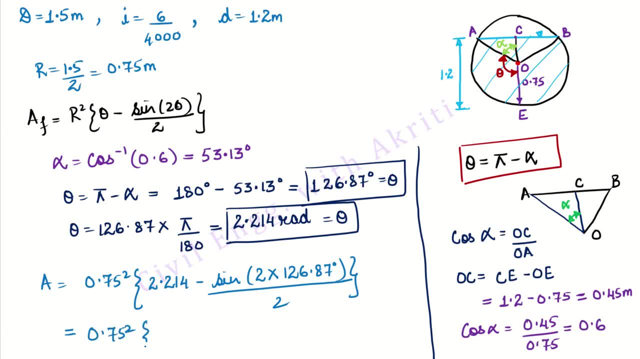 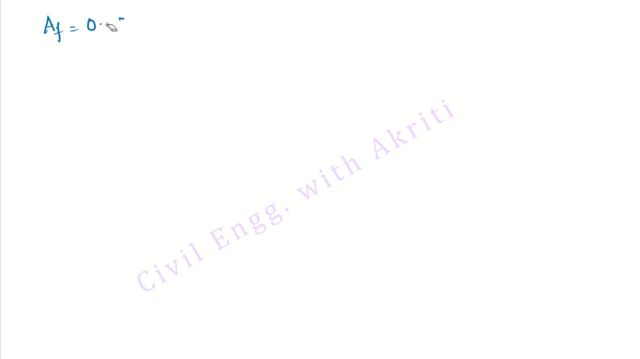 So if you calculate this, then 0.75 square into 2.214 will be equal to minus of minus 0.480.. So here minus into minus will be plus, So I can write 0.75 square. 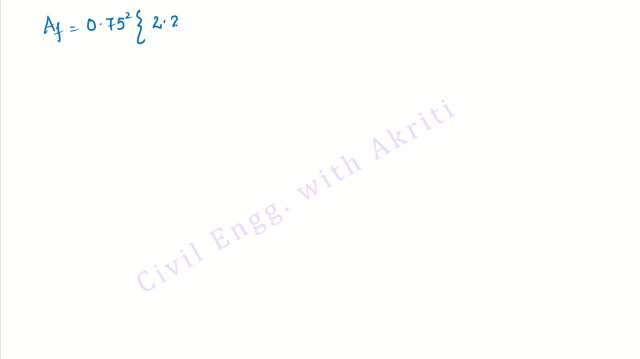 into 2.214, minus into minus of 0.48.. So minus into minus will be plus, So I can write 0.48.. So this area calculates to be equal to 1.515 m square. This is the area of flow. 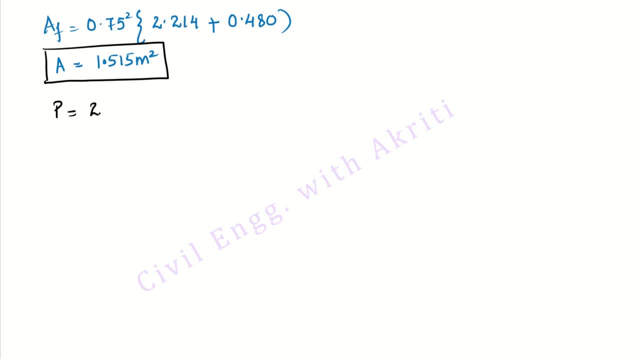 Now let's talk about perimeter. So perimeter is equal to 2r theta. So here theta will be in radians. So 2 into 0.75, into 2.214 is equal to 3.321 meters. so this is the value of perimeter.